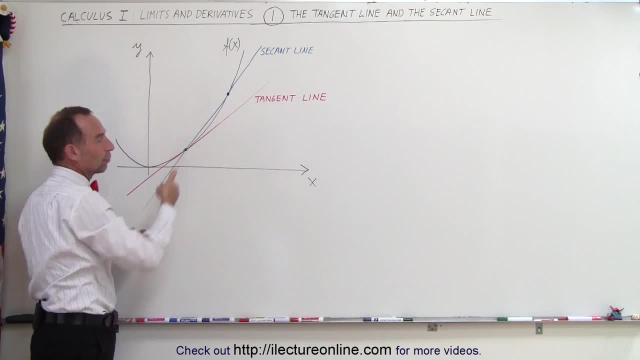 In other words, the secant line cuts across a function, of course, that is in a graphical sense, so to speak, so that it touches the function in two places. A tangent line only touches it at one single point, right here, and none of the other points on the tangent line are at the same. 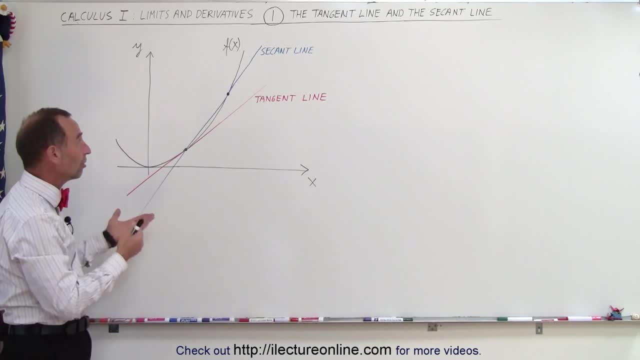 location as the function itself. So the difference between the tangent and the secant line is the tangent only touches the function once and the secant line touches the function twice. What we're going to see later on is we're going to see what happens. 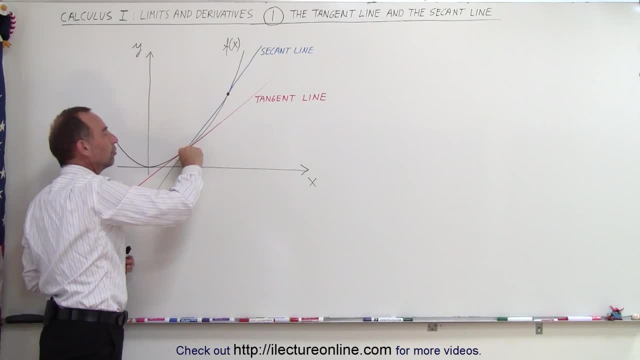 when you bring the second point closer and closer and closer to the first point, then you can see that the slope of the secant line will much more align with the slope of the tangent line and eventually you'll see that if we bring this point really close together, that the slopes of both 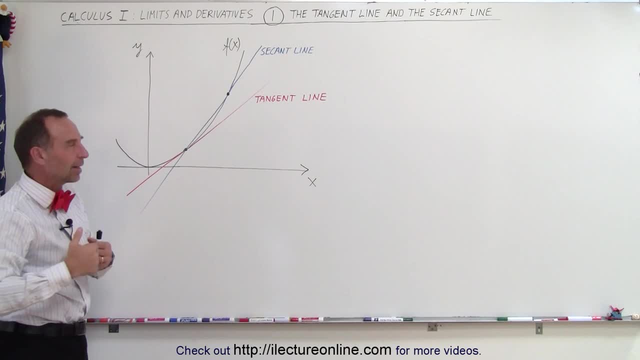 lines will be very, very close to one another, and that's the concept that, at least, will lead us to the concept of a derivative. So, if you understand what we mean by the tangent line, the secant line will be very close to one another, and that's the concept that we're going to talk about when you. 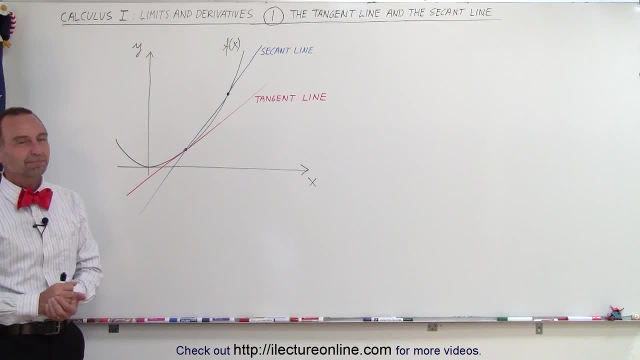 later on we'll talk about it in more general terms. So that's our start on looking at limitives and derivatives. 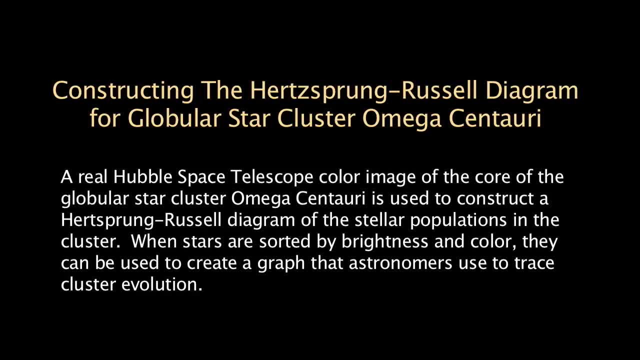 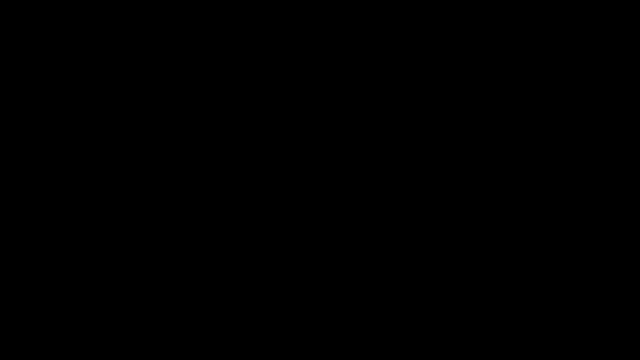 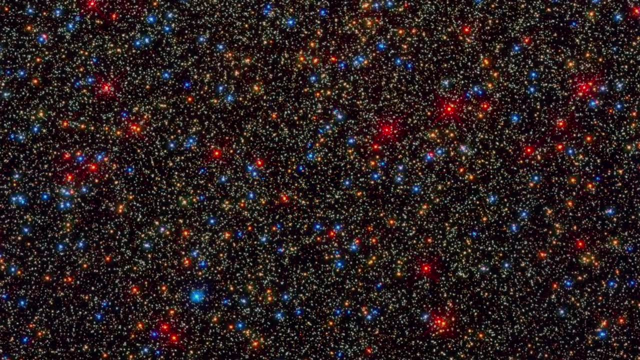 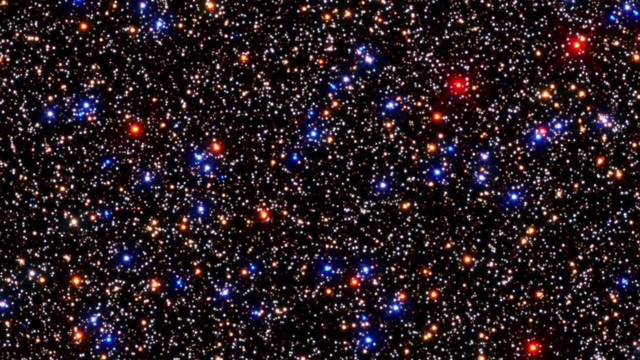 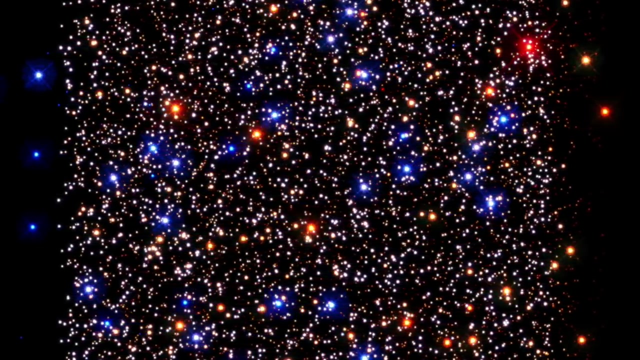 This is a Hubble Space Telescope image of the crowded core of the globular cluster Omega Centauri. The brilliant colors of the stars are real. They correspond to stellar temperatures. They can also be used to trace stellar evolution. Astronomers like to know how blue the blue stars are and how red the red stars are. so 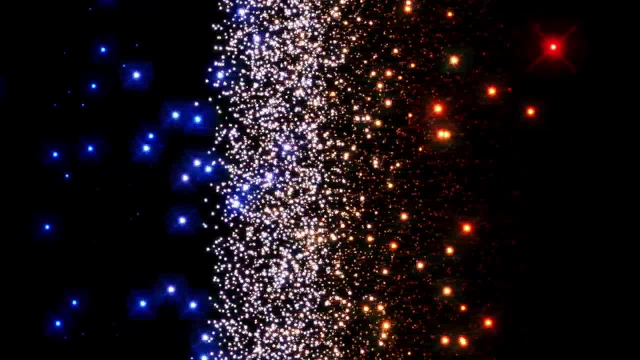 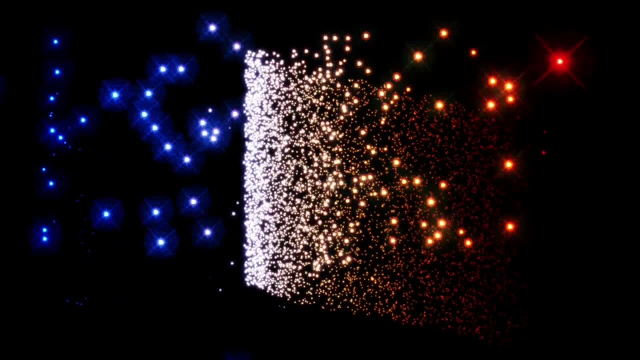 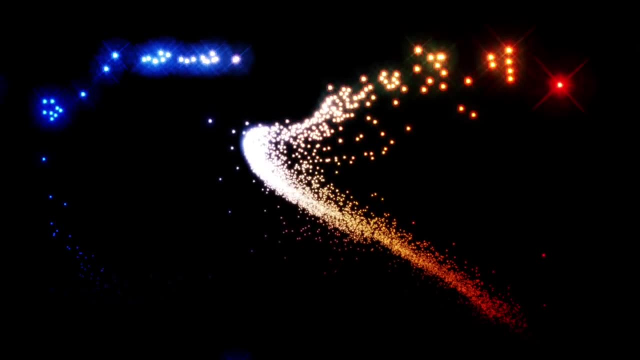 we'll first sort these stars out by color – blue on the left and red on the right. Next, we'll sort the stars according to brightness – the brightest stars at the top and the faint stars at the bottom. The final plot you see represents different stages of evolution of stars. Stars spend.